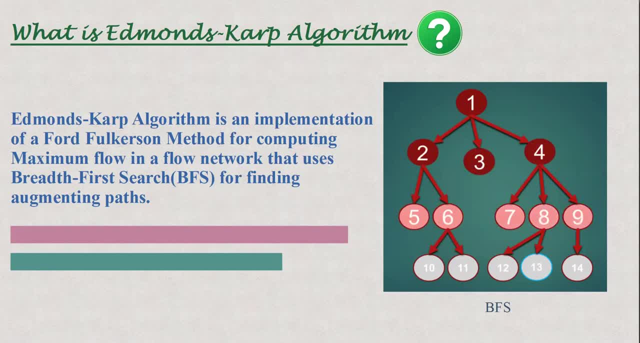 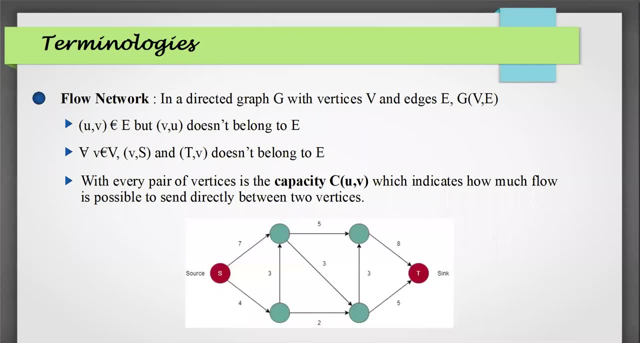 using dfs. Here is the given tree which shows how dfs works: Terminologies. Before moving to port focus method and Edmonds-Karp algorithm, let's have a look on different terms that we are going to use. First is flow network: A flow network in a directed graph that 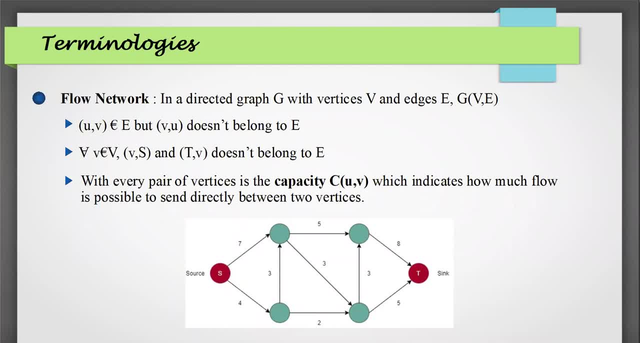 has source and sink t where belongs to e and does not belongs to e. that simply means that the flow is in one direction. Here we will have special vertices in the graph. that is, source s, from where the flow network starts, and sink t where it terminates. All the other nodes are called internals. 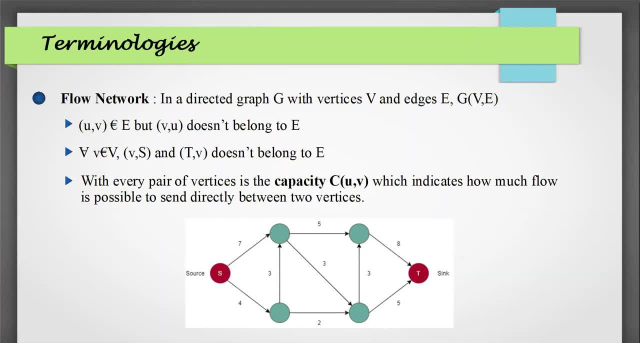 For all small v belongs to capital, V, v, s and t. v does not belong to e. This means that there are no outgoing edges from the sink and incoming edges to the source With every pair of vertices is the capacity which indicates how much flow is possible to send directly between the two vertices. 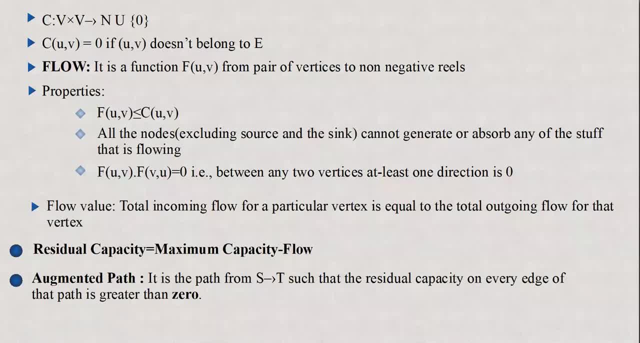 Capacity are non-negative If the capacity between two vertices is equal to zero means that there is no edge u comma v that belongs to e, or there is no flow possible between the two nodes. Flow it is a function from pair of vertices to non-negative deals It is the actual unit of flow that take. 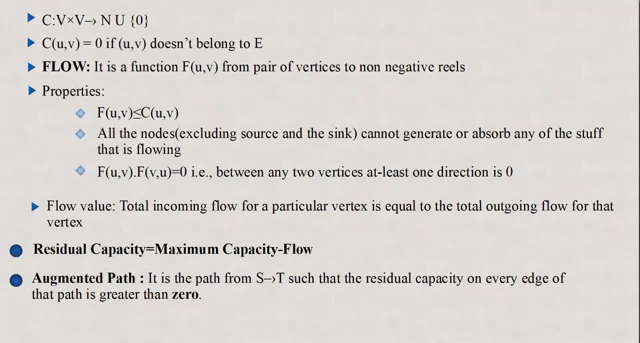 place between the two nodes, Flow is always less than the capacity between the two vertices. Internals can't generate or absorb the flow. F into F is equal to zero, which simply means that there is only one direction possible and at least one of the direction is zero. Flow value: Total incoming flow is equal. 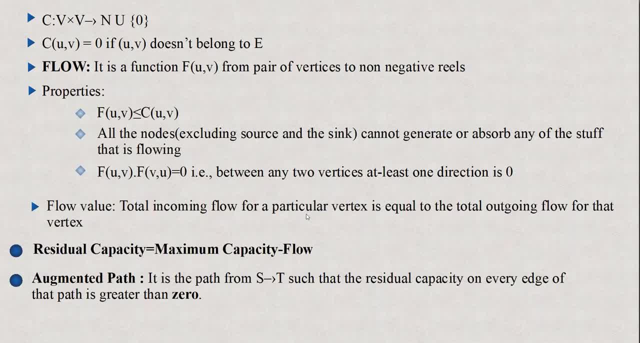 to total outgoing flow for the vertices. Residual capacity. Residual capacity is the remaining capacity between the two vertices After the flow has been augmented through that path. residual capacity is equal to the maximum flow minus flow Augmented path. It is the path from source to the 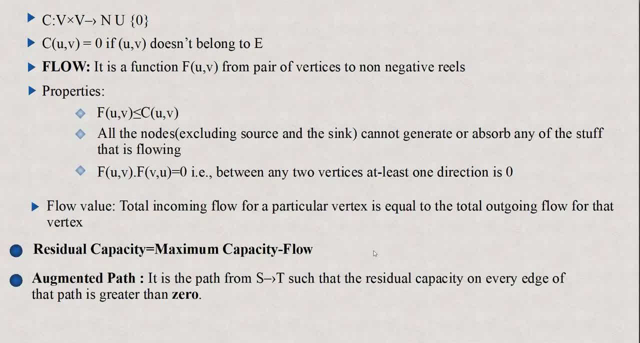 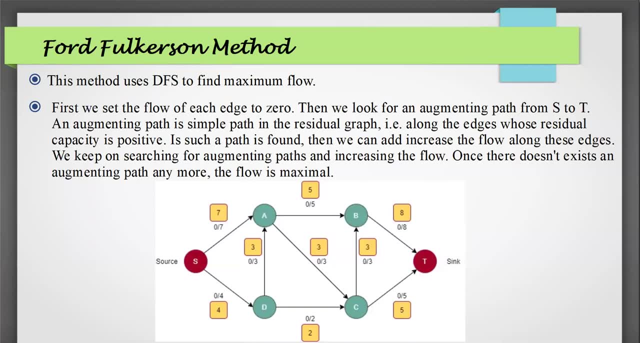 sink such that the residual capacity of every edge along that path is greater than zero. Now we discuss the Ford- FWOOSball method. It uses DFS to find the maximum flow In this given flow network. we will- We will- initialize flow as 0 and maximum capacity between the vertices is given by 0-7, which 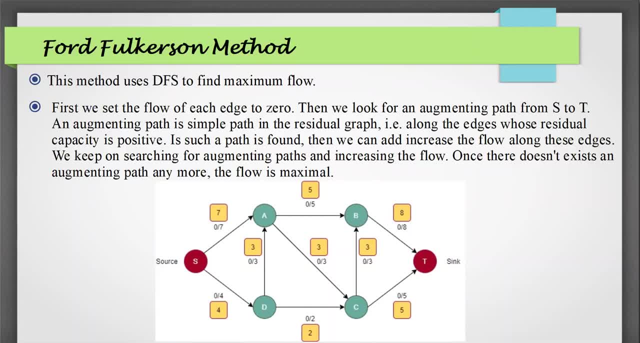 means that 0 is the flow and 7 is the maximum capacity. here it is given in this graph from S to A. Residual capacity is equals to maximum capacity, since the flow is 0 initially. Now we will find all the possible augmenting path and repeat until no augmenting path are. 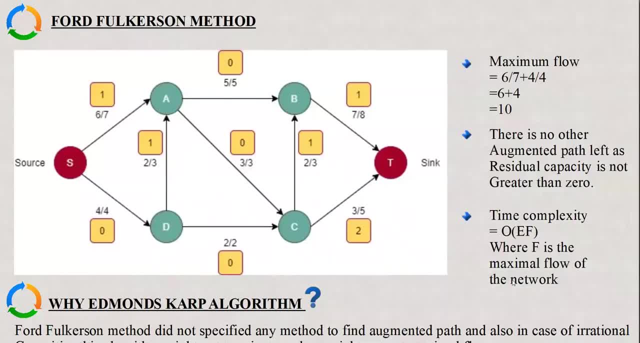 left. Finally, we will get the given flow network. Maximum flow is equals to 6-7 plus 4-4, which is equals to 10, where 6 and 4 shows the flow, while 7 and 4 shows the capacity between the two vertices. 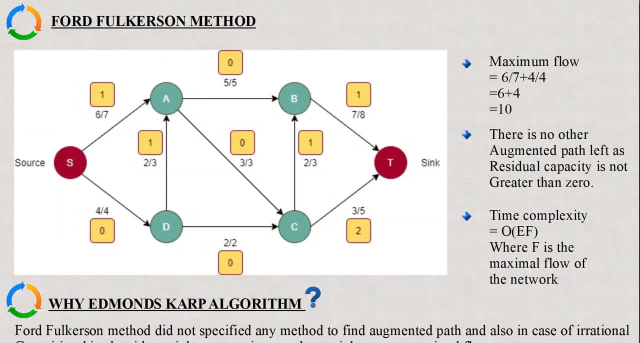 There is no other augmenting path. Time complexity is equals to order of EF, where F is the maximum flow. Why Edmonds-Karp algorithm? Because this method did not specify any method to find augmenting path and also in case of irrational capacities, this algorithm might not terminate and we might not get the maximum. 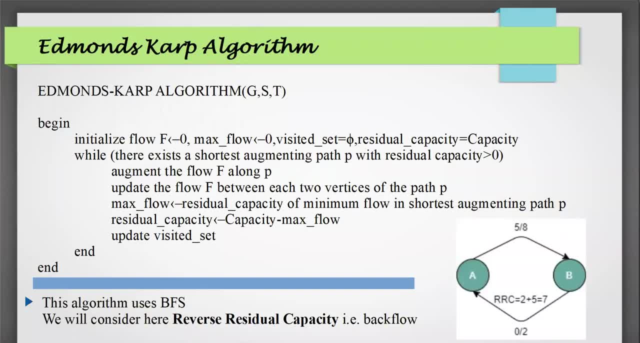 flow. Here is the algorithm for Edmonds-Karp method to find the augmenting path. Firstly, we will initialize flow. Maximum flow is equals to 0 and visited set, residual capacity, S capacity and null set. While there exists a shortest path- P- with residual capacity greater than 0- we will follow. 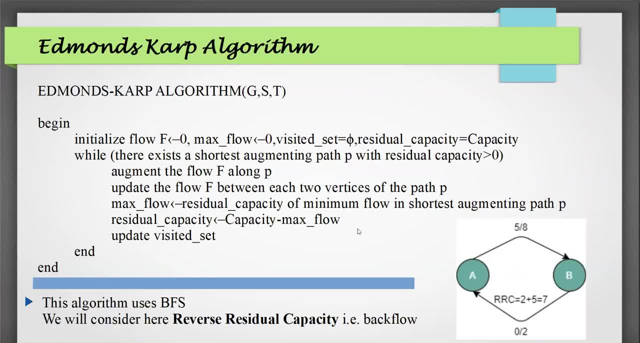 all this process and then we will later terminate the algorithm. Here we will also consider the reverse residual capacity, ie the backflow, In the given figure A to B and B to A. Here in the given figure from A to B and B to 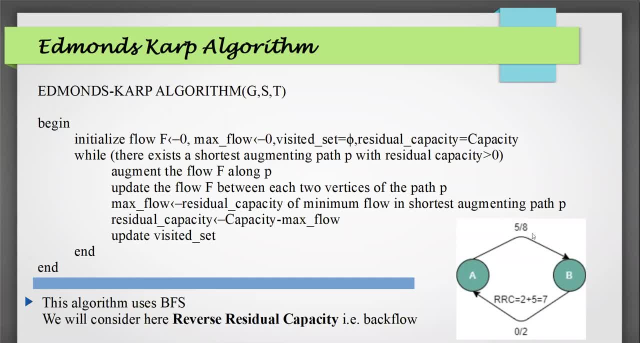 A flow is 5 and 8 is the capacity from B to A. 0 is the flow and 2 is the capacity. So reverse: residual capacity is the capacity from A to B and the flow from B to A, So reverse. 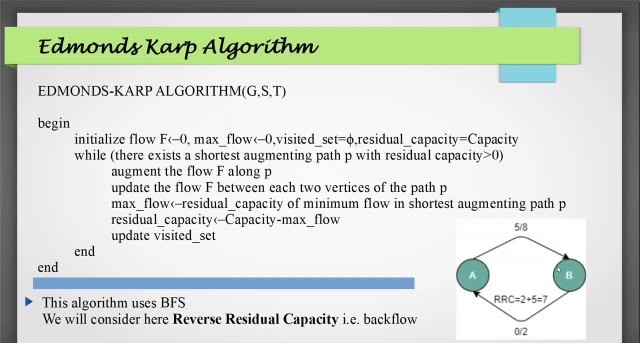 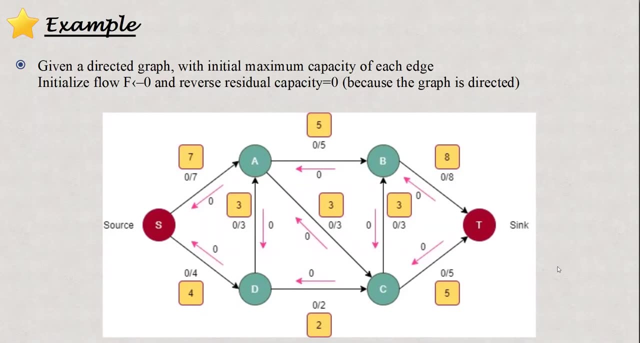 residual capacity is 2 plus 7, which is equals to 7.. Because we can stop moving that 5 units of flow from A to B In this given example, we are given with the initial maximum capacity and we will initialize the flow as 0 in the first step. 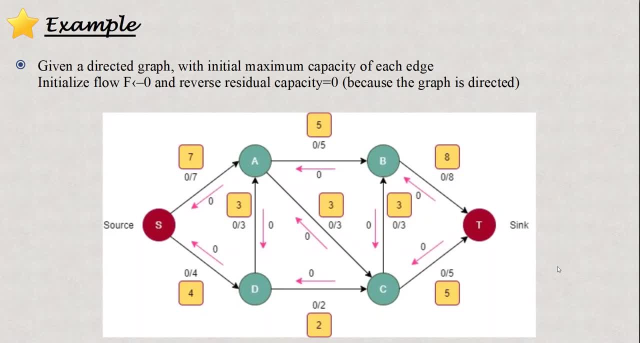 So we will have the network as given here, where the digits in yellow box is represent the residual capacities between the 1 and 0.. So we will have the network as given here, where the digits in yellow box is represent the residual capacities between the 1 and 0. 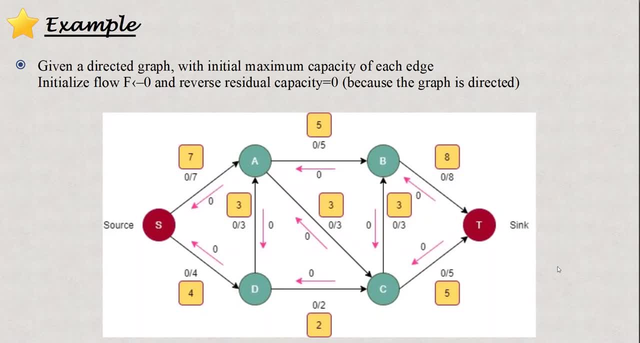 So boom, Aha. We have visited the total and past conventions of operation. In the latter one we have encuentraру to view all the step can noodle which the frequently used foraying organization. Now we need to find the augmenting paths in the sq. 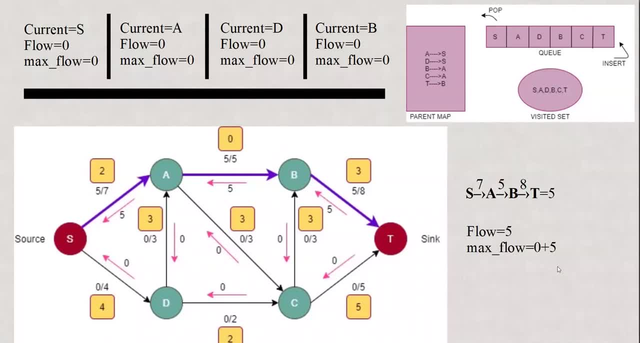 In the next step we will insert the elements in the cube and the visited node in the visited set. So we already have the first step. When we see it, we have our elements in the sq. Firstly, we will visit the source s, so let us put that element into the cube here. 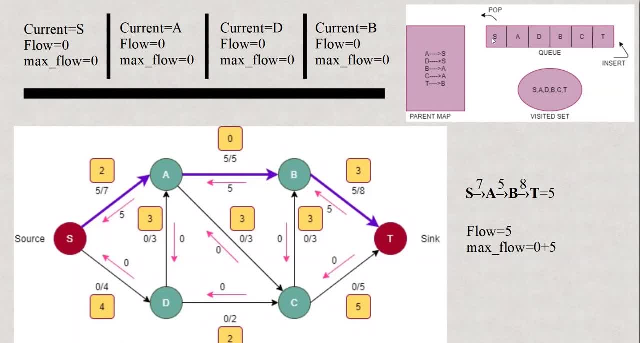 Now let us pop element from s in the cube. So after popping out the element from the cube And then check again, after placing in element element exercise here: element in the мотрt we will have current is equals to s. so now the neighbors of s are a and d, which are not visited. 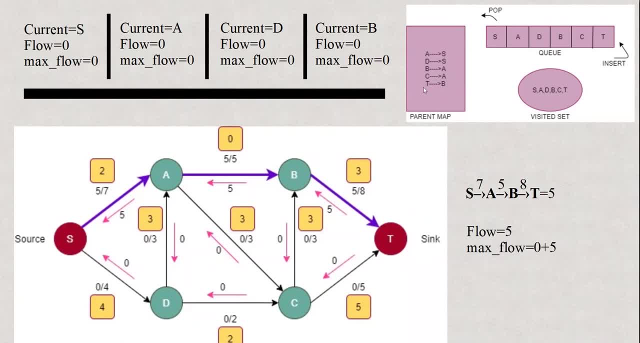 and have the residual capacity greater than zero. so we will add these elements, a and b, to the visited set as well as in the cube. simultaneously we will update the parent set by saying that a was visited through node s and d was visited through node. our current now becomes a after. 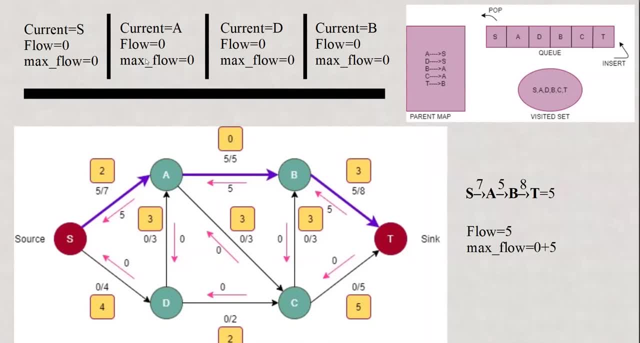 popping the second element from the cube. current now becomes a after popping the element from the cube. so now we will see the neighbors of a that are d, c and b. but from a to d we have reverse residual capacity as zero, so we can't consider this as zero. 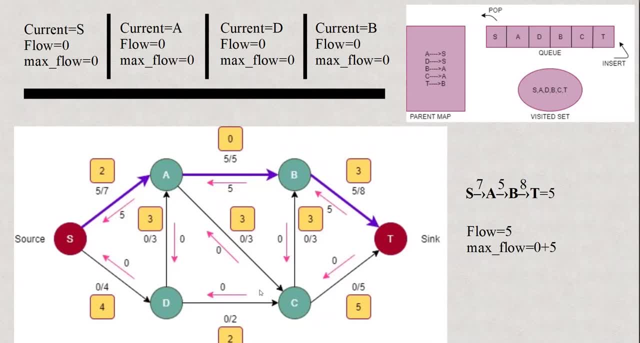 a path. so we are only left with two of the options, that is, B and C, that have residual capacity greater than zero, as well as they are not visited. so we will put B and C into the queue as well as in the visited set, and we will 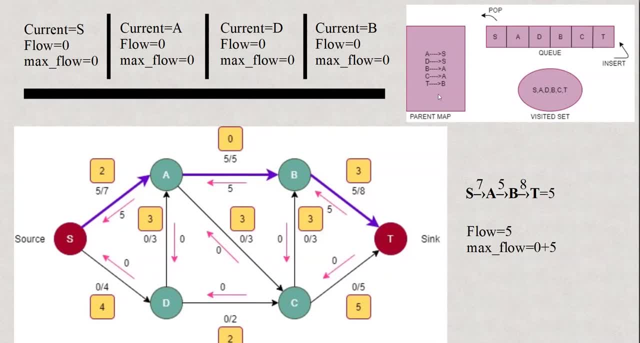 simultaneously update the parent set by saying that B got visited through A and C also got visited through A. now we will pop up the element D from this queue. now D does not have any neighbors whose residual capacity is greater than zero and which is not visited. so now let us pop out element B from the queue, so we have the. 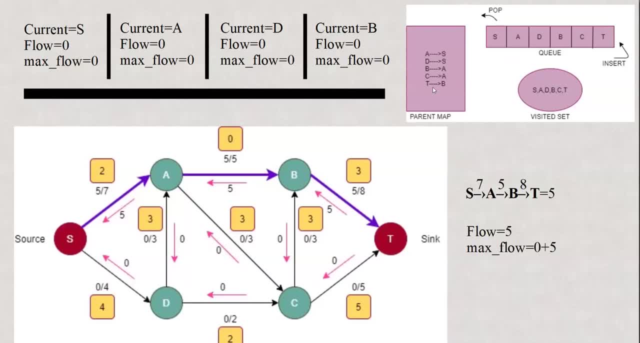 neighbor T. so now we can update the parent set by saying that T got visited through A- B. now we will backtrack this parent map to get the flow. so T got introduced by B, B got introduced by A and A got introduced by S. so the augmenting path here is S- A. 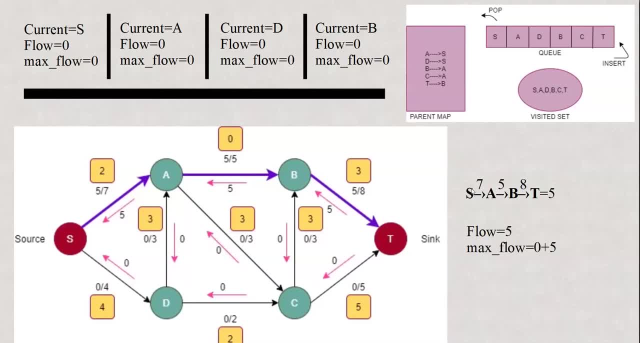 B and T and its respective flow are 7, 5 and 8. so the maximum flow possible through this path is 5. so we will update the flow value as 5 and max flow is equals to 0 plus 5. so now given here is updated flow after finding the first. 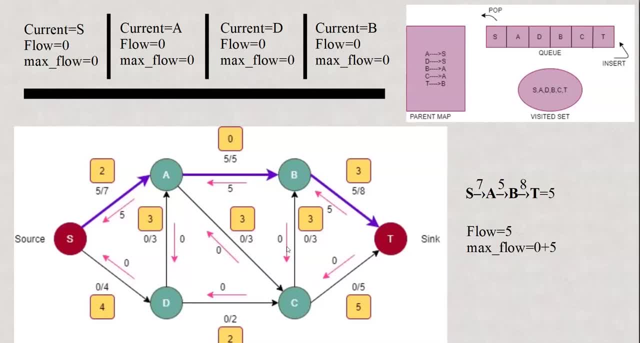 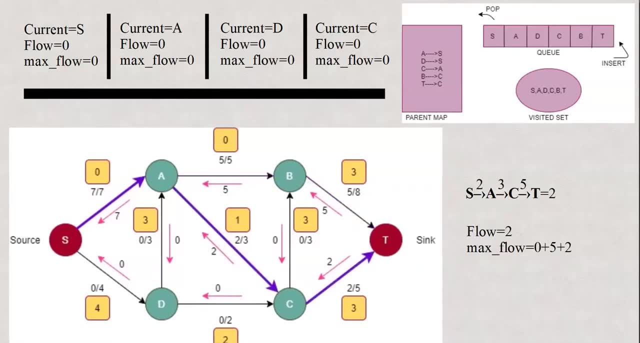 augmenting path flow is updated, reverse flow is also updated and residual capacity along this path is also updated. we will again follow the same procedure to find the another augmenting path. elements in the Q will be S, then A, then B, then C, and then C and B, which are neighbor of A, and we will have T, which is neighbor of C. 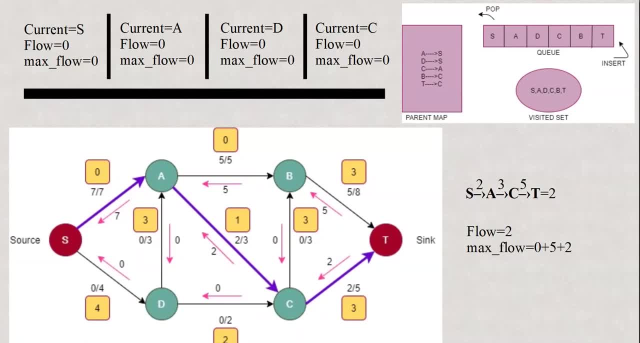 Simultaneously we will update the parent map as follow: A got introduced by S, B got introduced by S, C got introduced by A, B got introduced by C and T got introduced by C. We have the path as follow: S, A, C and T by backtracking. 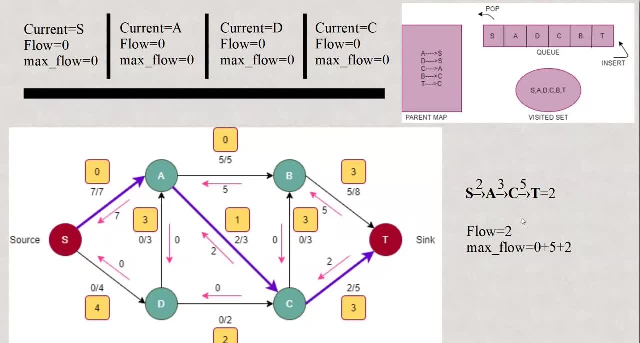 Maximum flow through this path is 2.. Therefore, flow is equal to 2 and max flow is equal to 0 plus 5 plus 2.. We will update the flow residual capacity and reverse residual capacity along this path. This is an updated graph given here after the second iteration. 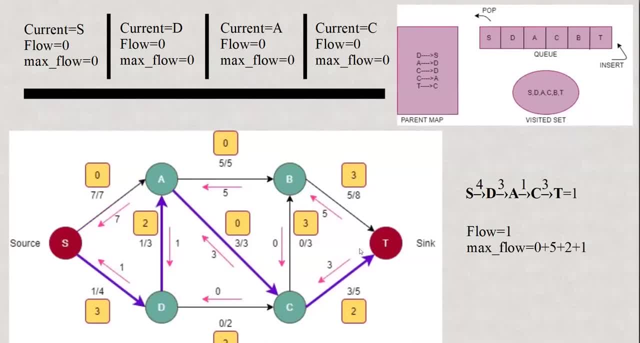 Follow the same algorithm again to get the augmenting path as S, D, A, C and T. Maximum flow through this path is clearly mentioned here as 1.. So flow is equal to 1 and max flow as 0 plus 5 plus 2 plus 1, and update the flow network as shown here by adding the flow to the path S, D, A and C. 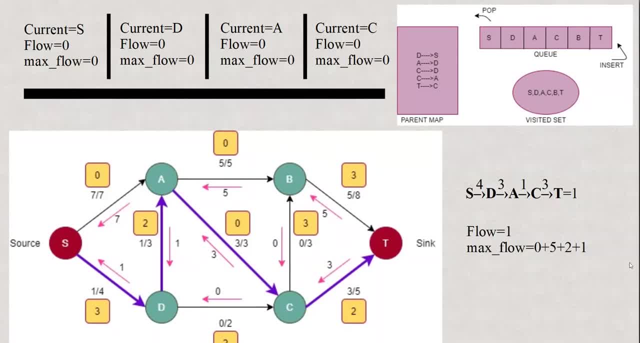 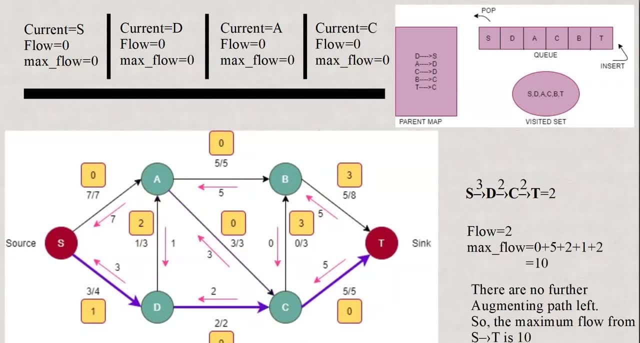 Updating the residual capacity by the formula residual capacity is equal to capacity minus flow and simultaneously update- reverse residual capacity. If the value of figure of S, D, A, C and T is equal to 0, maximum flow here is 0.. 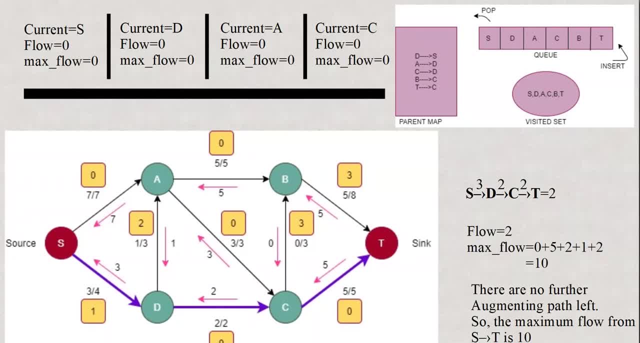 Follow the same step as we have done before and find the augmenting path with a residual capacity greater than 0, which is S, D, C and T, and flow that is possible here is 2.. So maximum flow here is 0 plus 5 plus 2 plus 1 plus 2, which is equals to 10, and there are no further augmenting path left as the residual capacity for S, D, C and T is not 0. 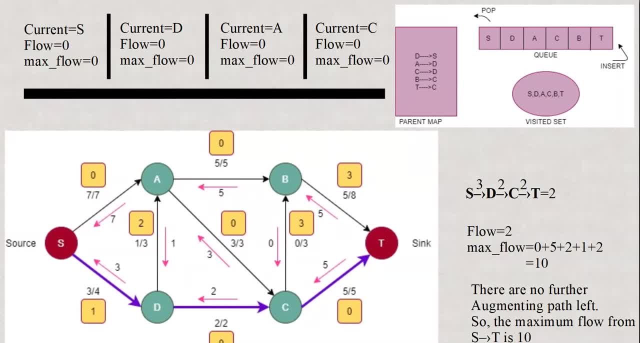 every possible path is 0.. So 10 is the maximum flow and the augmenting paths are S D C T, S D A C T, S A C T and S A B T. 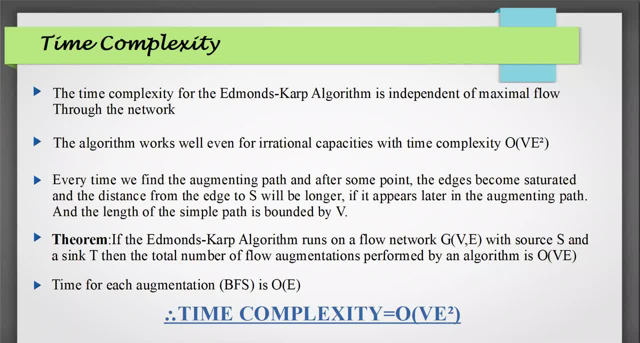 Now let us discuss about the time complexity for this algorithm, which is equals to order of V E square. It is independent of maximal flow. According to the theorem, this algorithm runs on a flow network with source S and sink T, Then the total number of flow augmentation performed is of order V E. 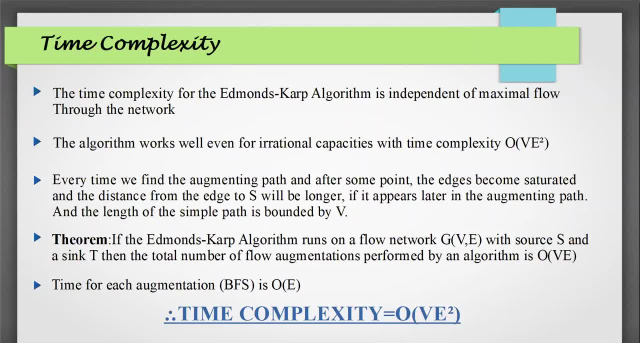 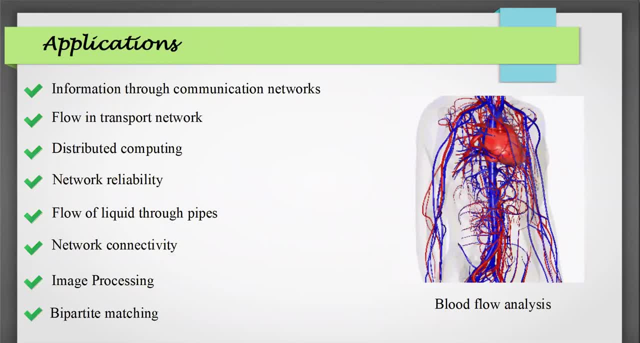 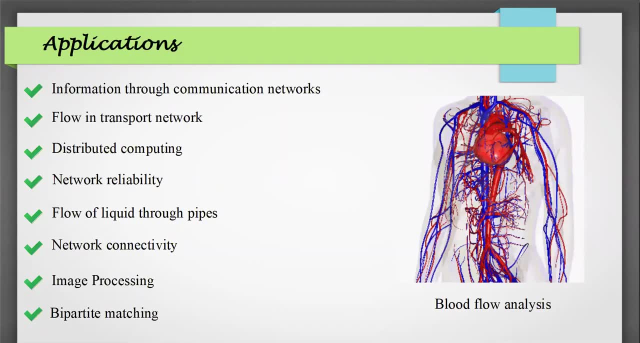 And the time for each augmentation BFS is order of E. Therefore the time complexity is order of V E square Applications. Here are some of the applications of Edmunds' gap algorithm, Like blurred flow analysis, flow of liquid through pipes, image processing, data mining, flow in transport network and many more.